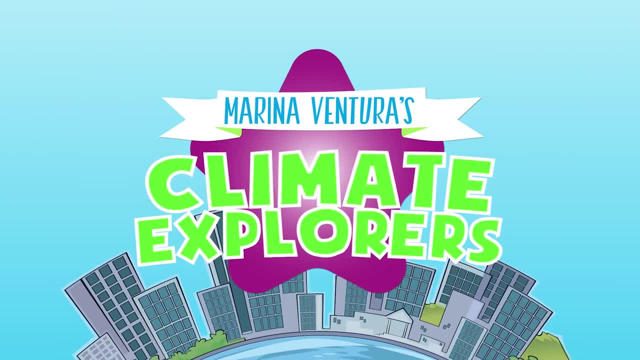 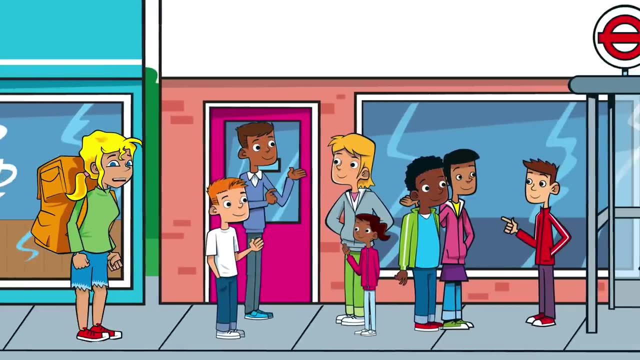 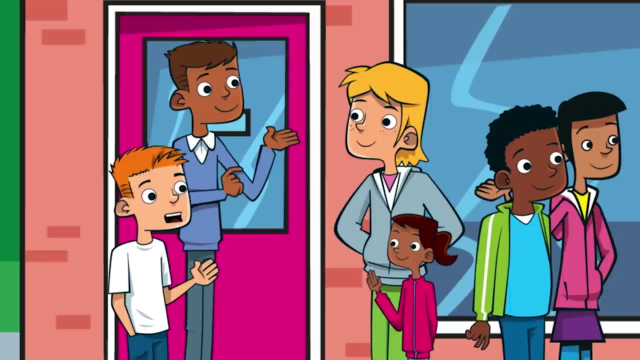 Marina Ventura's Climate Explorers. Now, we all like talking about the weather. In fact, people in Britain are well known for it. The weather's quite good, It's quite hot And it's quite sunny, Windy and very cold, A bit rainy, Freezing. 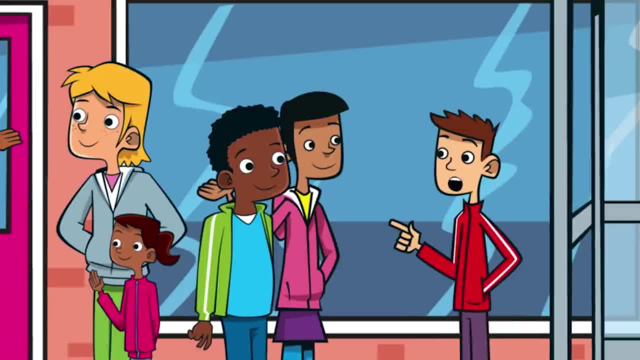 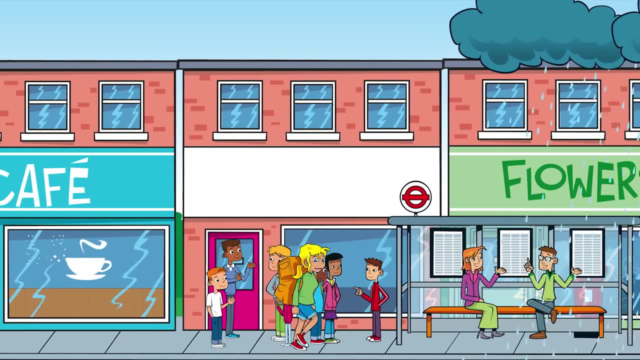 About a bit sunny, Very windy. All of the leaves are falling off the trees. Talking about the weather is one of the ways we start conversations, especially with people we don't know. One of the reasons for this is because it's something we have in common with everyone around us. 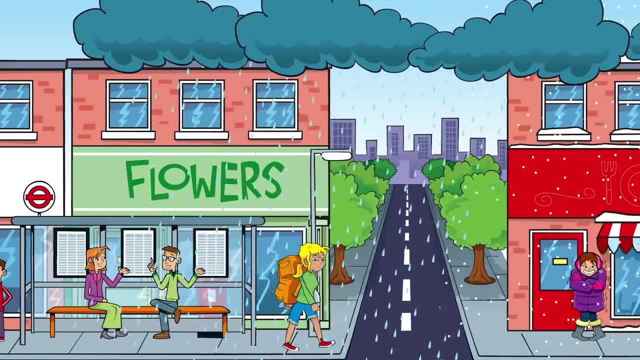 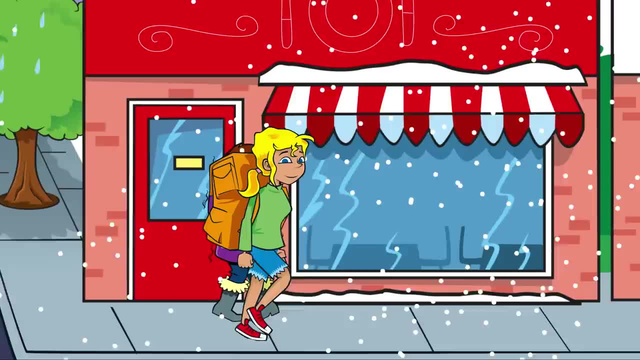 If it's a rainy day and I get soaked in a downpour, you might have got wet too, And if it's freezing cold, then you're probably feeling it as well, And weather is a topic that everyone has an opinion about. Maybe it's chillier than it was yesterday. 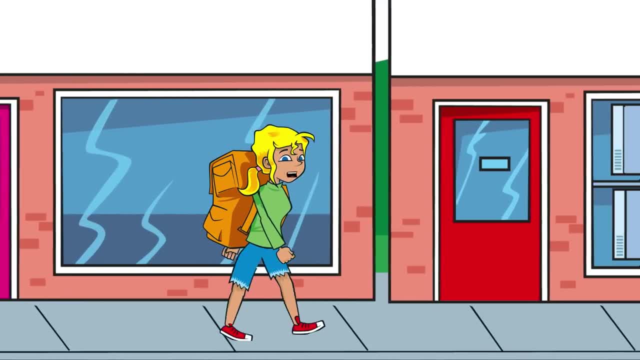 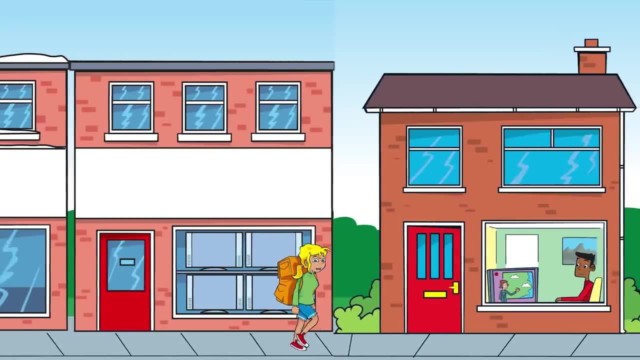 Perhaps you didn't expect to need a coat, because you thought it was going to be a bit warmer. Not knowing quite what to expect means it's often sunny. It's surprising. That's why people like to read, listen to or watch weather forecasts every day. 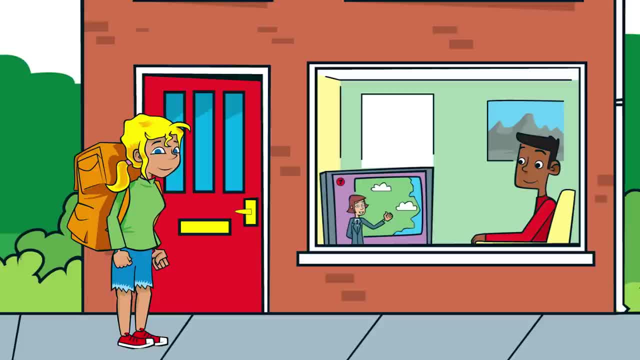 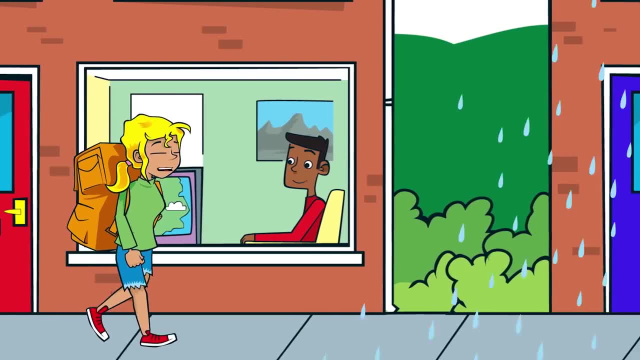 To help make sure they've got the right clothes on, And, with rain heading down south, tomorrow is set to be wet, so don't forget your umbrella. After all, no one likes getting soaked, But weather's quite a strange thing, Even if it's cold and wet on one day. 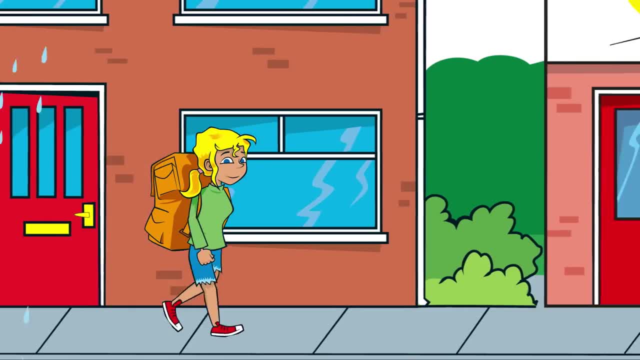 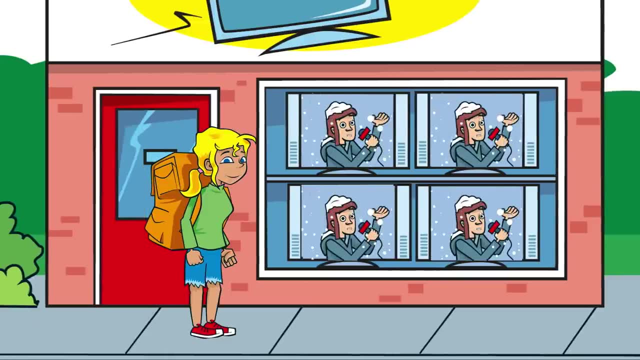 the next day can be very different And not everyone gets the same weather, even when they're in the same country. Schools in the north of England will be shut today due to heavy snow, But in the Midlands there's no snow, so schools are open as usual. 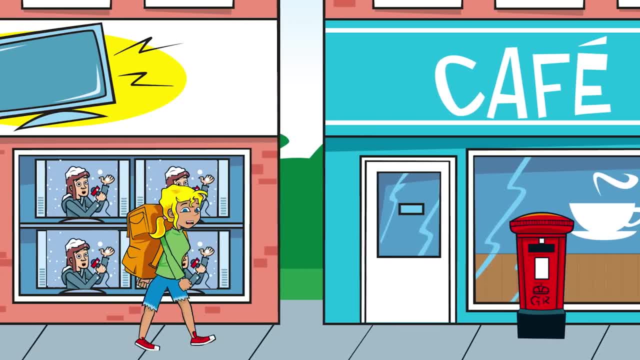 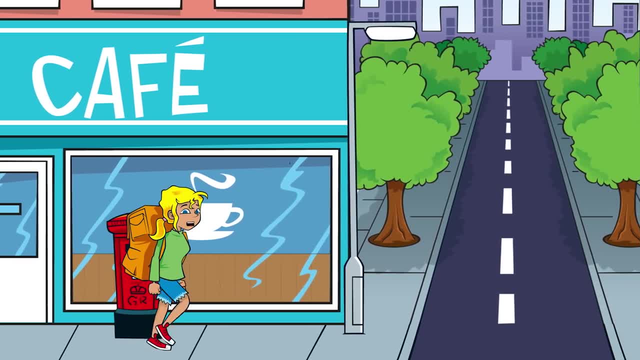 Sorry, kids. So, as you can see, weather is constantly changing, Which is probably why it's so interesting. As we've seen, weather forecasts help us to know what to expect, But even without them, we have a feeling about what the weather should be like at different times of the year. 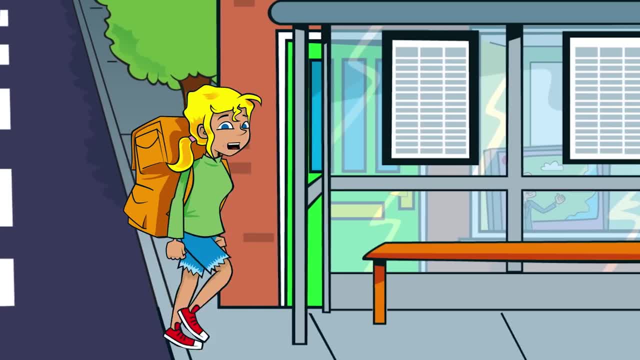 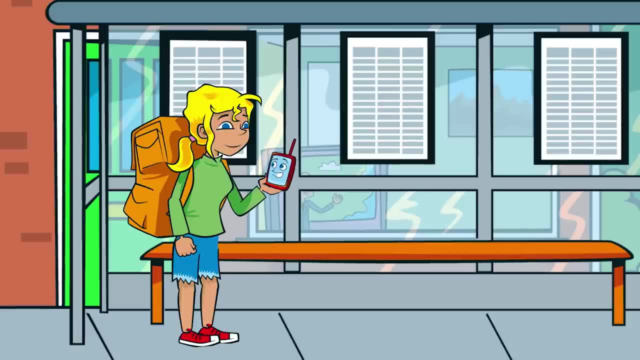 We expect it to be cold in winter and warmer in summer. Have you ever wondered why this is? Let's find out. Let's ask Map App. He's great at explaining things. It's all to do with climate. There's a saying: weather is what you get and climate is what you expect.